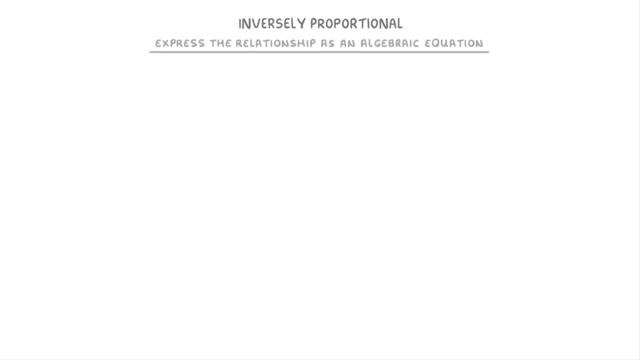 Another thing that we can do is express the relationship as an algebraic equation. The key thing to understand for this is that saying that the time taken is inversely proportional to the number of farmers is exactly the same thing as saying that time taken is proportional. 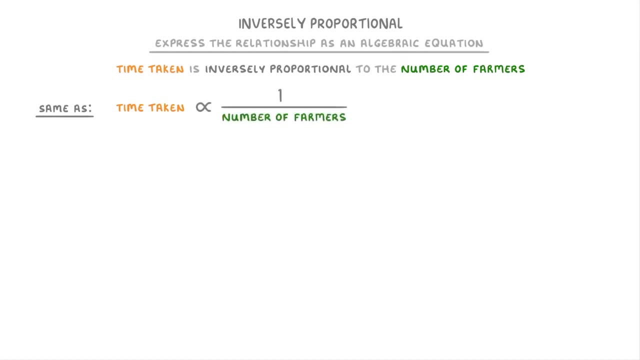 to 1 over the number of farmers. So if we let time taken be t and the number of farmers be f, then we'd have: t is proportional to 1 over f. To write this as a proper equation, though, we need to change the proportional sign to: 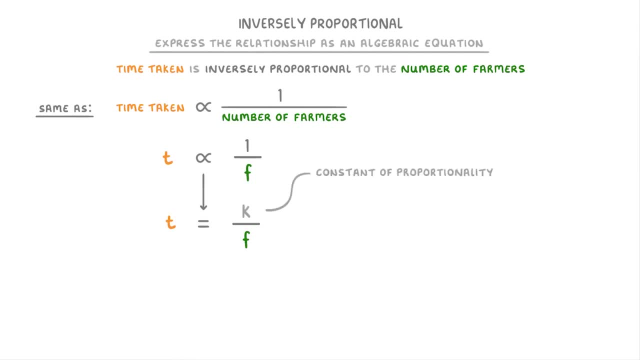 an equal sign, And to do that we have to include a constant of proportionality, which we normally show with the letter k. It's up to you where you put the k, but we normally put it in the top right of the equation, like we have here. 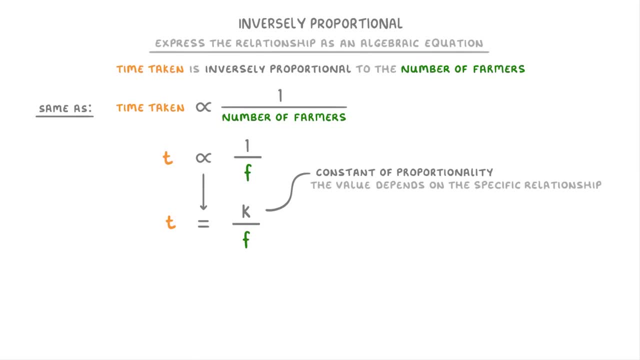 Now, the particular value of k depends on the specific relationship, so could be anything like 0.4,, 8, or whatever. If we pretend that in this case it was 8, though, then, as you can see, we now have an equation. 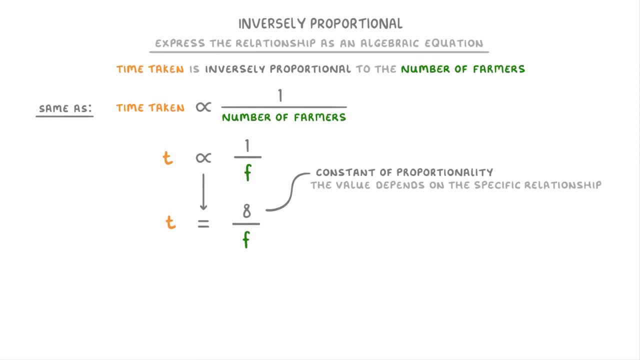 that we can use to convert between time taken and the number of farmers. For example, if there were 2 farmers then f would be 2. So we could put the 2 into our equation and find that time would be equal to 8 divided. 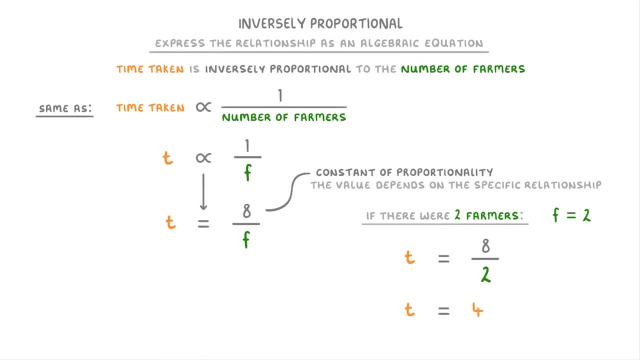 by 2. So it would take them 4 hours to pick all of the apples, Whereas if there were 5 farmers then we'd do- t equals 8 over 5, to find that it would only take 1.6 hours. 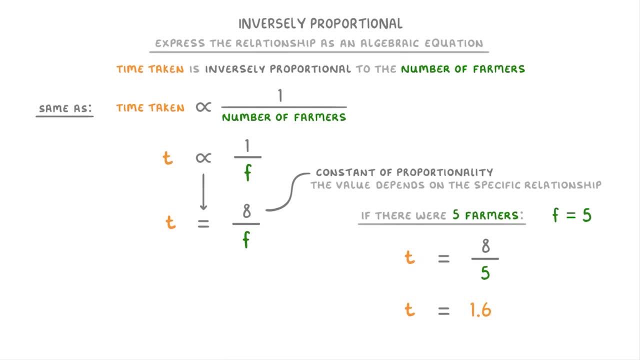 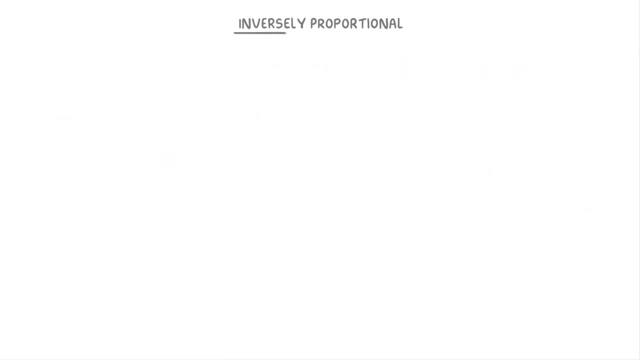 So because we had more farmers in this second case, it took less time to pick the apples. So to sum up this video: inversely proportional means that as one variable increases, the other variable decreases proportionally, And we can show these relationships on graphs which will always have this downward slope. 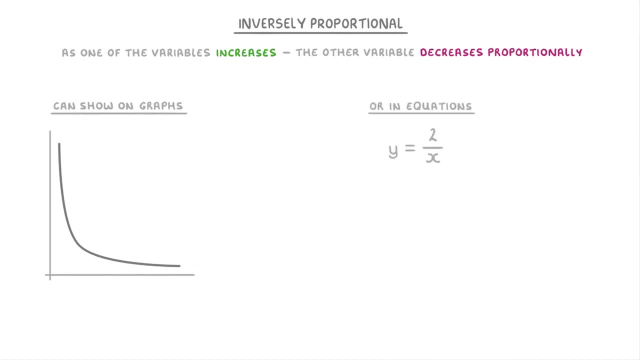 or in equations, for example, like y equals 2 over x, which will always have one variable equal, some number, which we call our constant of proportionality over the other variable. And one last thing to point out is that it doesn't matter if there are other numbers.